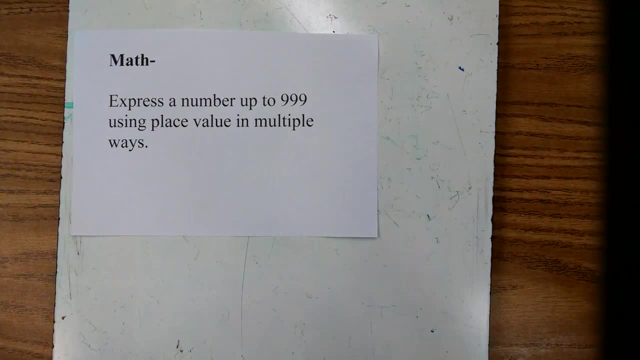 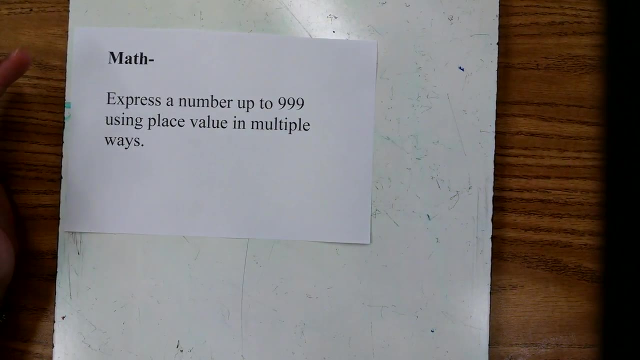 Hi guys, I want to go over something we learned today in school, and it is how to show or how to express a number up to 999 using place value in multiple ways, And, simply put, that means I can show a three-digit number by using different 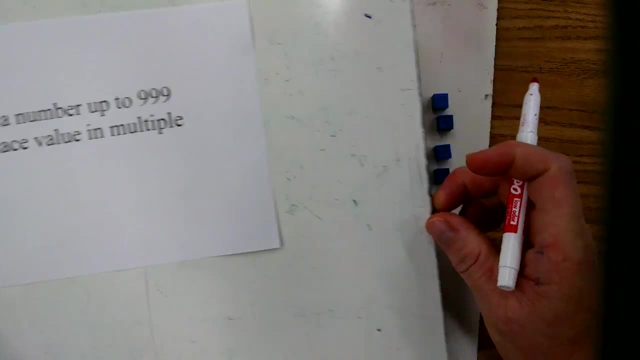 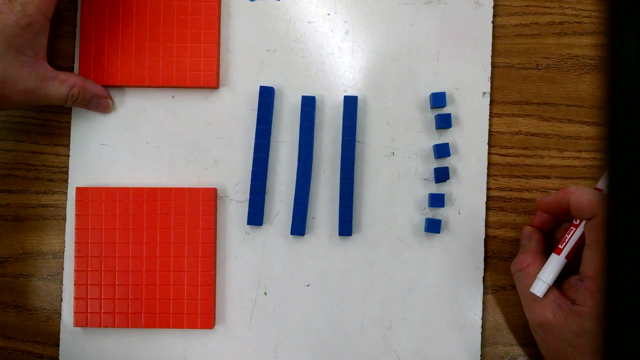 combinations of ones, tens or hundreds. So let's get down to it. What I've set up is 236, and the most common way that most people would go ahead and try to make make this using blocks would be by putting two hundreds, which I've done, and 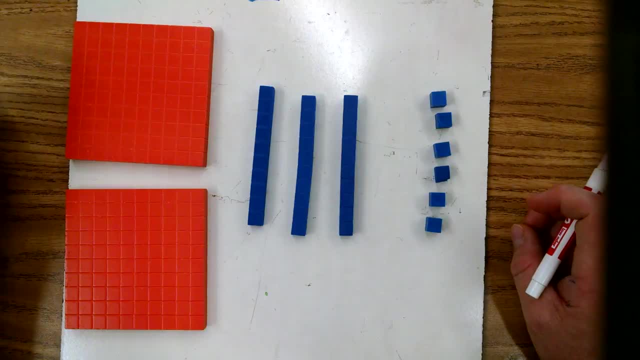 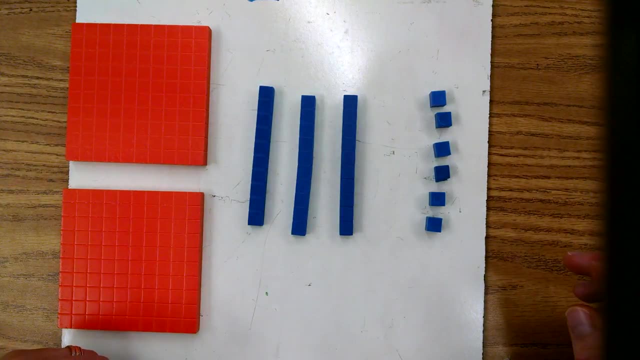 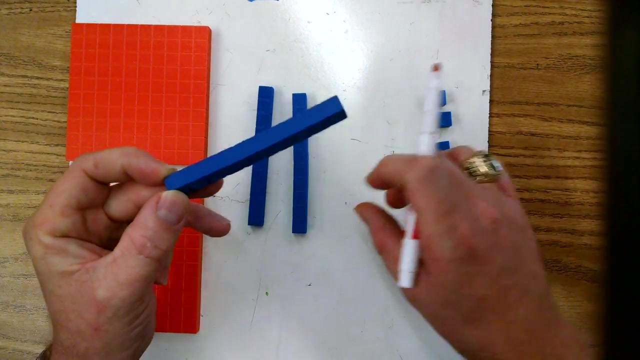 three tens and six ones. But there are many, many other ways, different combinations of ones and tens that we can, that we can use to to show this number. So let's start by trying to trade a ten in for ten ones And we don't call. 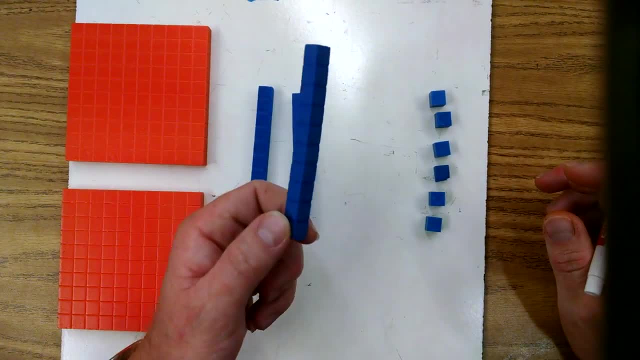 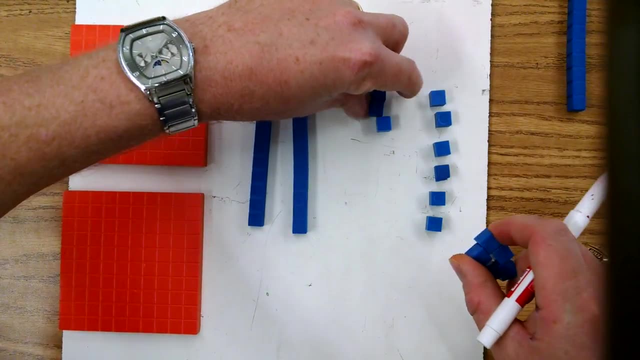 it trading so much anymore. the new terminology is decomposing, So we're going to decompose it or split it up into ten more ones, And I've got those ones right here. Now you can draw this out and I'll show you a bunch that I've already drawn. 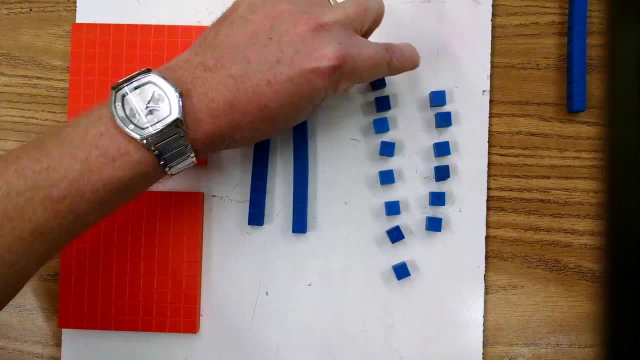 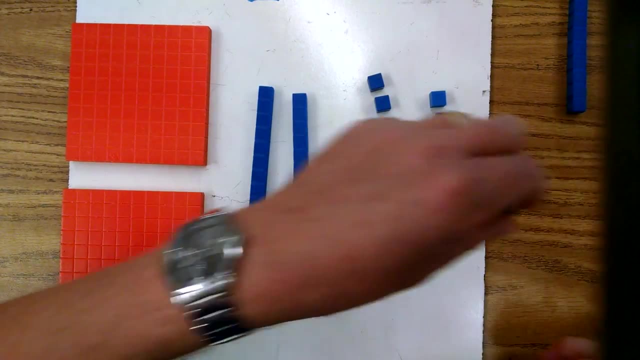 out ahead of time. But let's go ahead. and if you were going to draw them out, you want to make sure you draw the right amount, because otherwise you're going to get the wrong answer: 1, 2, 3, 4, 5, 6, 7, 8,, 9, 10.. So this time we still have our 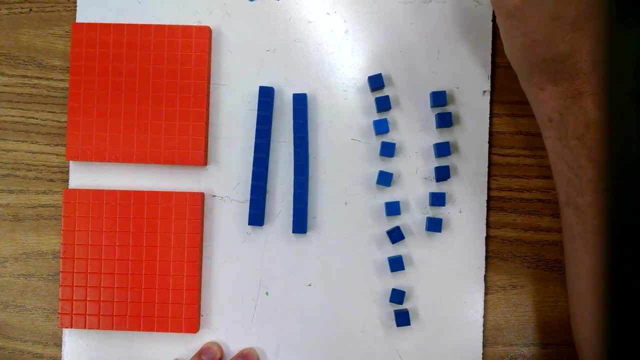 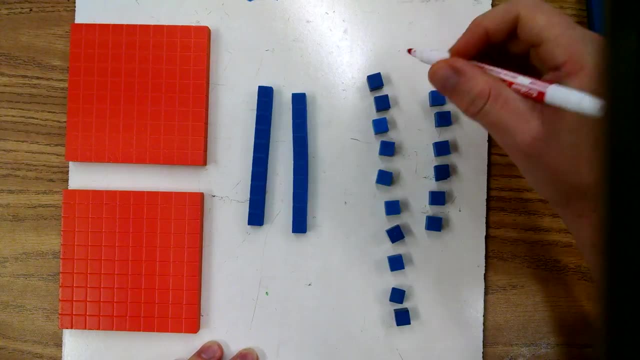 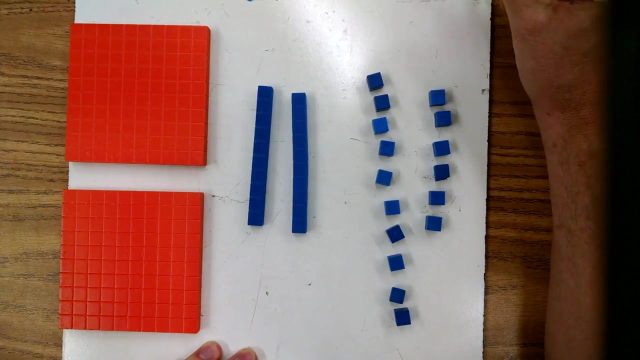 two hundreds. We have two tens this time instead of the three tens, And we have, that's, ten and six ones. Ten ones and six ones gives you 16.. So now we have 16 ones. See what happened. look at the difference between this one and this one. 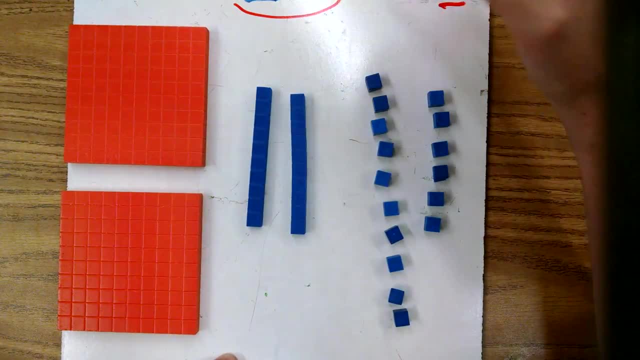 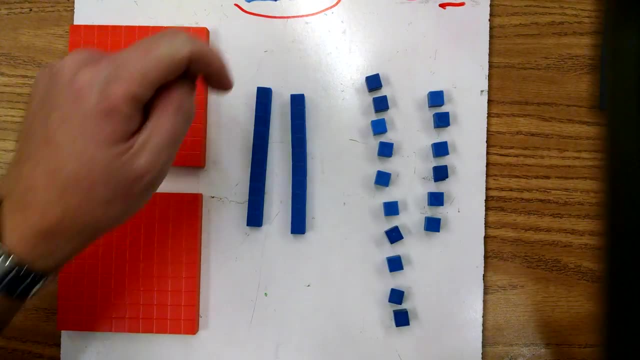 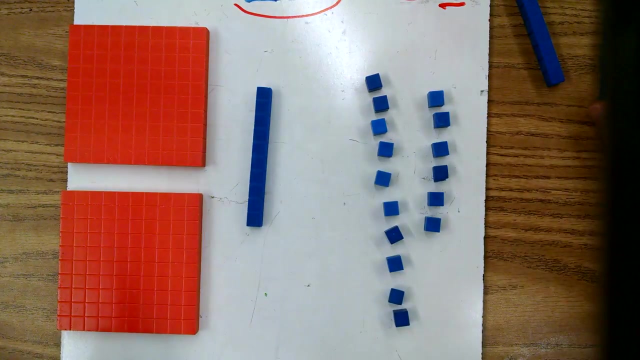 They both name the same number, but I'm using a different combination this time of ones, tens and hundreds. So the trick is it's gotta equal the same number number. all right, let's, can we go ahead and decompose this? sure, and we're going to go ahead. 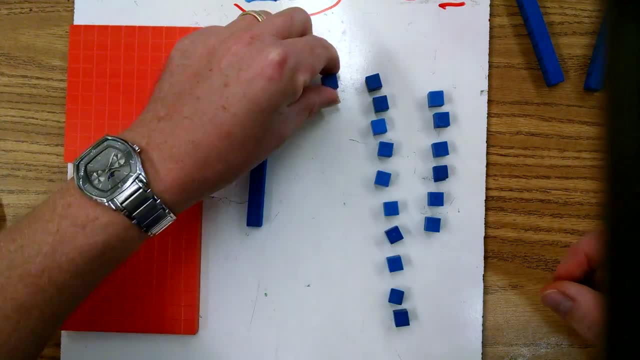 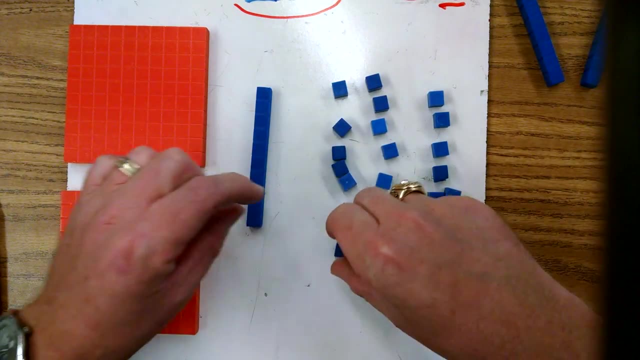 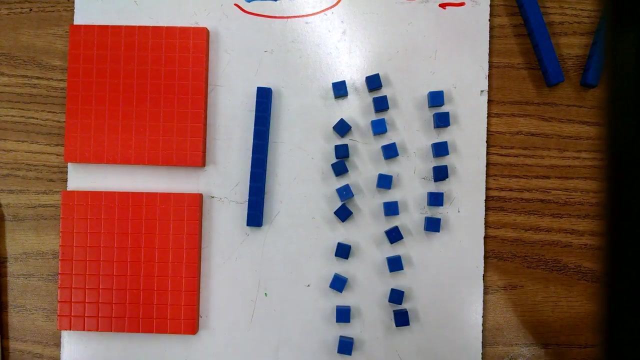 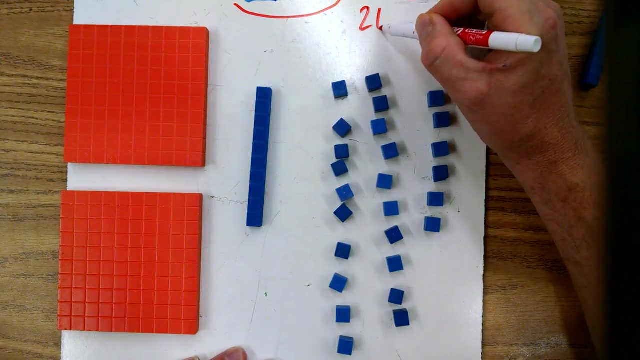 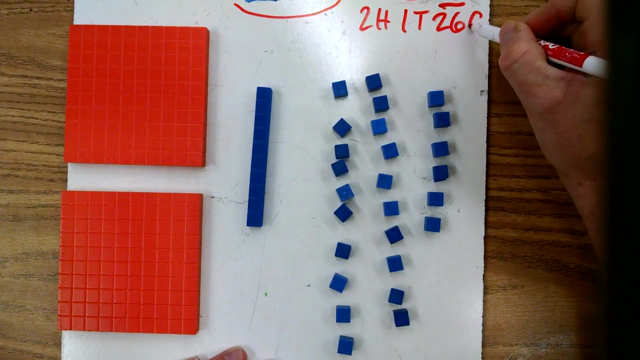 and do it into 10 more ones: one, two, three, four, five, six, seven, eight, nine, ten. so now we have a whole different combination here, but it's still the same amount, same number. so we still have our two hundreds, we have one ten this time and we have 26 ones. 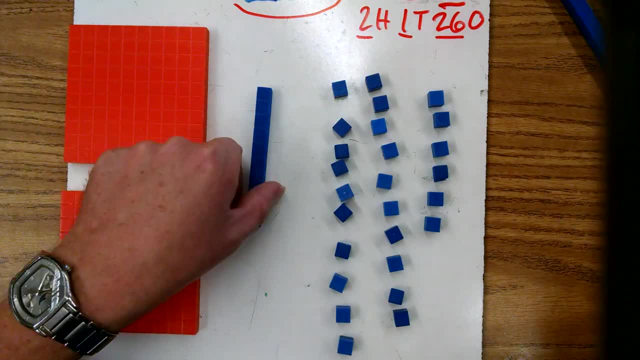 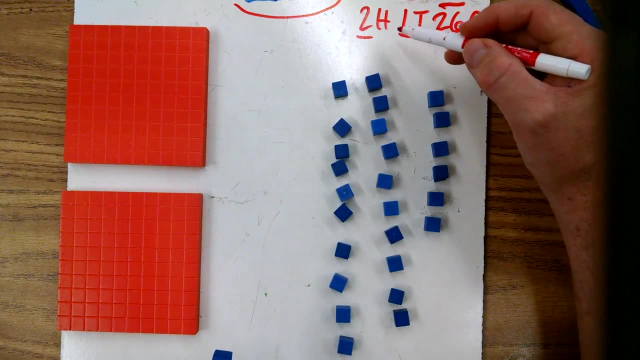 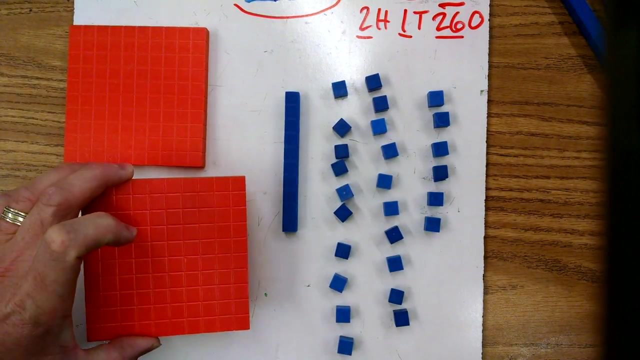 we could do the same thing with this and we'd have you got it 36 ones, and we would have zero tens that time and still our two hundreds. but just for the fun of it, let's leave our 10 there and let's come over here and do you think we could? 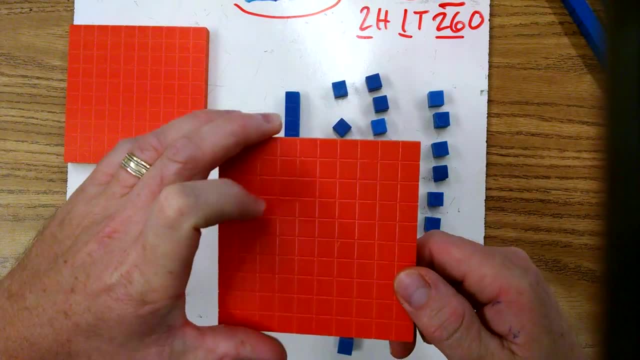 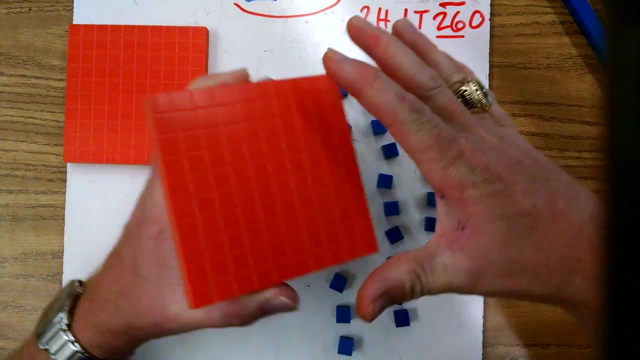 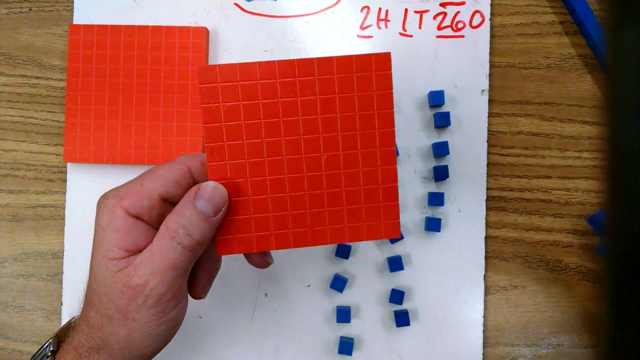 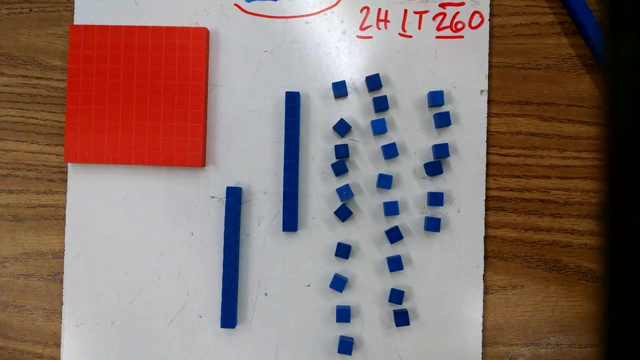 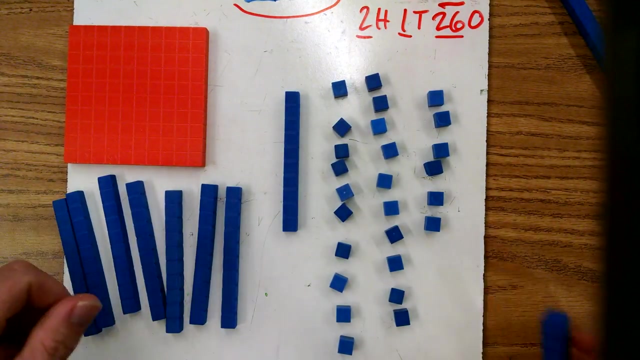 decompose one of these you would. you want to trade it in and decompose it, break it apart into a bunch of single units, a hundred units. can you picture a hundred units- that's a lot to count. so i'm just thinking: why don't we break it up into 10 tens, right? so let's do that. one, two, three, four, five, six, seven. 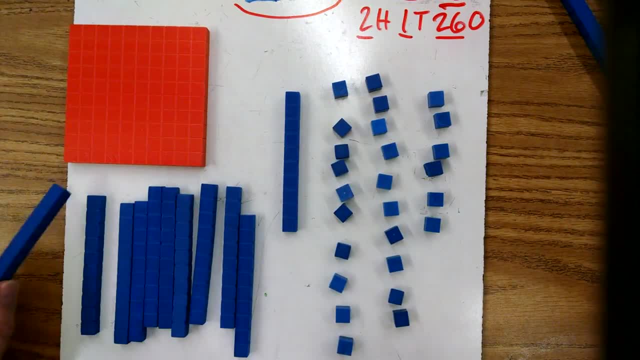 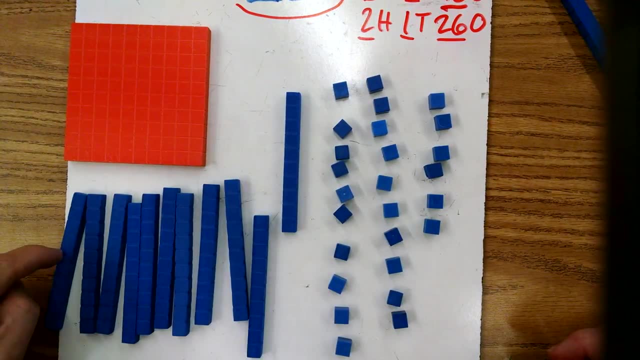 eight, nine and ten. now, if these were all spread out on your paper, you could always count them out and circle them as a hundred, couldn't you? 10, 20, 30, 40, 50, 60, 70, 80, 90, 100, 110, so you could circle. 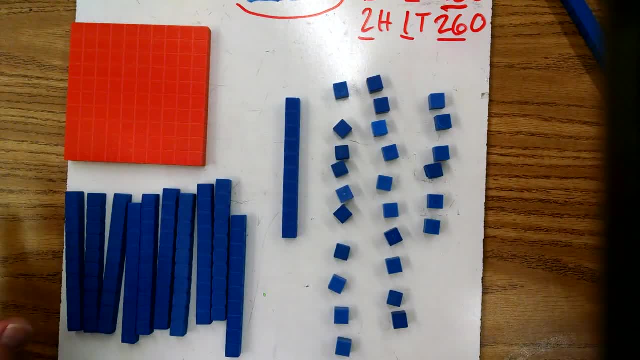 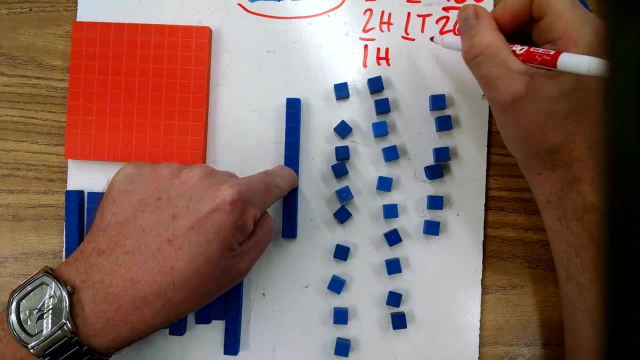 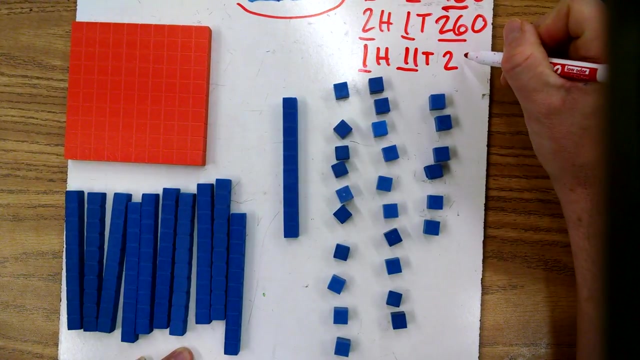 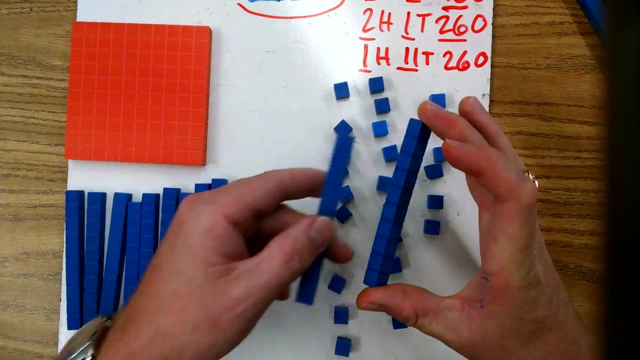 that and group it into a hundred. so now that's a whole different combination. now we have 100, we have 10, 11 tens and those 26 ones. Now those are just a few ways We could trade this and this. I mean we could trade them all for whole different combinations. 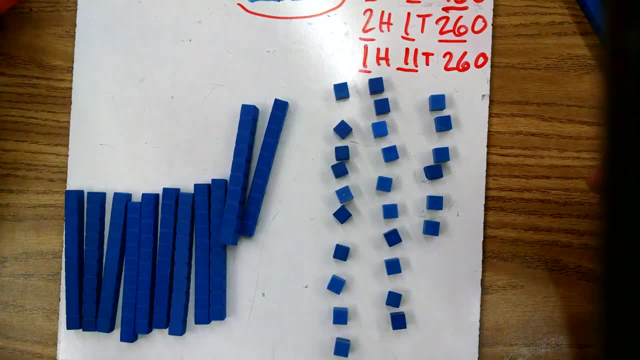 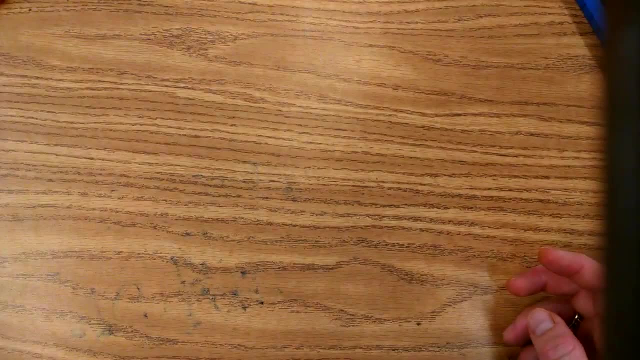 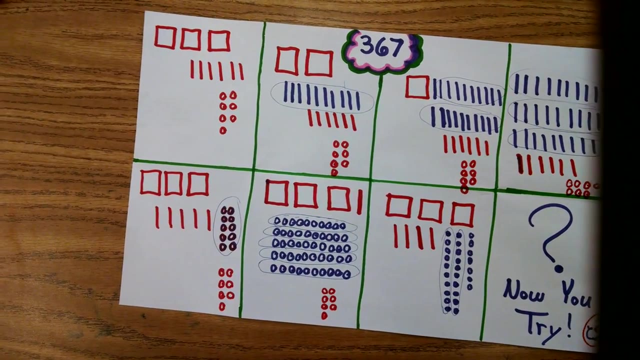 If we want to trade this in for 10 tens, then we'd have a whole different combination. What I've done is I've pre-written a whole page so you can get an idea of just some possibilities, And then you can try one on your own.